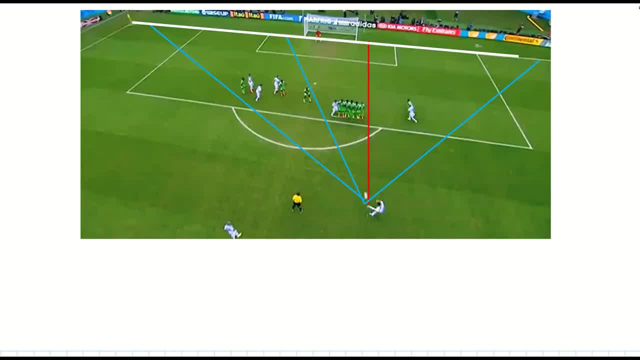 to give you a bit of background before we get into doing an example. So in this picture here you can see that the person here is taking a free kick and there's many, there's infinite amount of waves that that football can get to this white line. The shortest way is going to be. 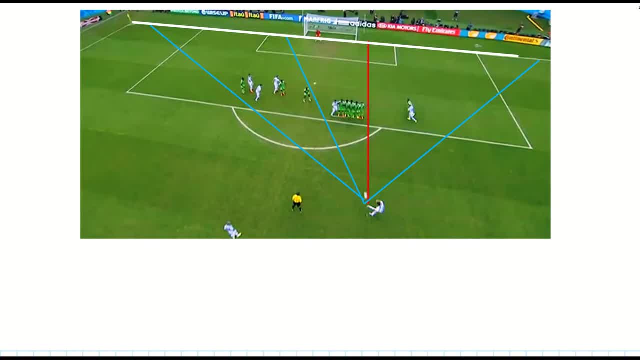 by following this red line, and if we follow this red line, what's happening here basically is that it's creating a 90 degree angle at that white line. So we said there's infinite lines, it can take all of these blue lines, but the red line is the shortest distance and it will create that. 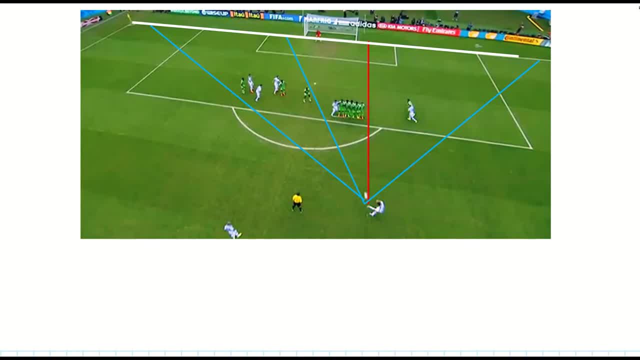 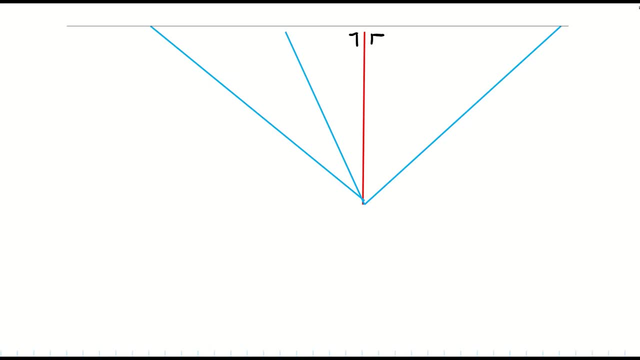 90 degree angle when it hits that white line. So here you can see it when it's sketched out. So the shortest distance is the shortest distance and the longest distance is the longest distance. The shortest distance is that red line when it creates a right angle at the line that we're 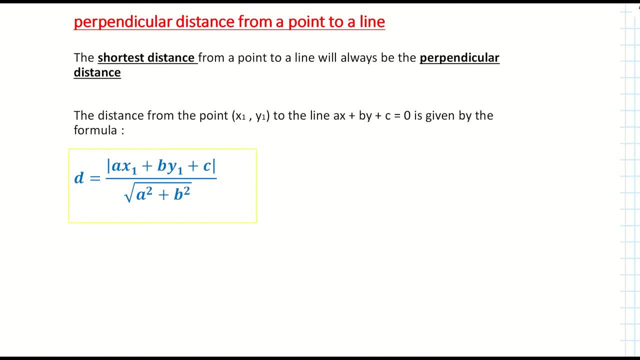 trying to get the distance to. So, before we get to our example, the formula is written down here from our log tables on page 19.. A couple of pieces of information you just need to be careful with once again is that the a, b and the c are what you're subbing into your formula Now. the a 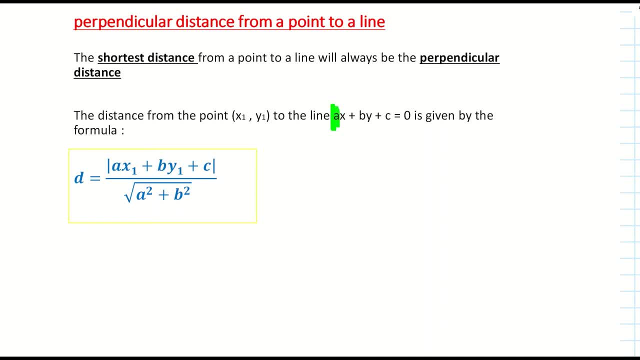 is the number that's in front of the x. in the equation of the line. The b is the number in front of the y. The y is the number that's in front of the y. The y is the number that's in front of the. 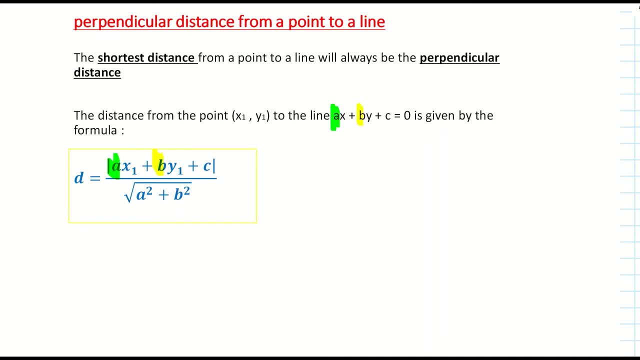 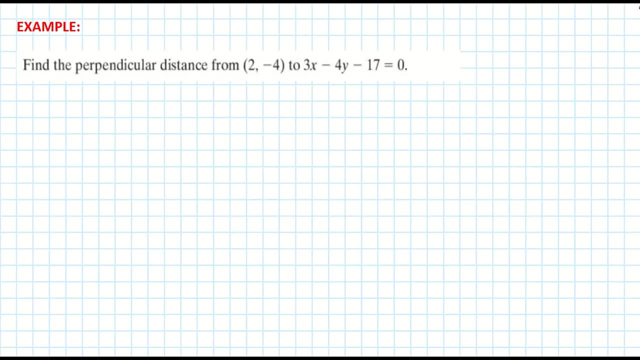 y from our equation, And then you have your c, which is the number on its own, the constant, the c, And they're the three numbers that you're going to have to sub in to your perpendicular distance formula. So let's go and do an example. So this example from our texts and tests is asking us to 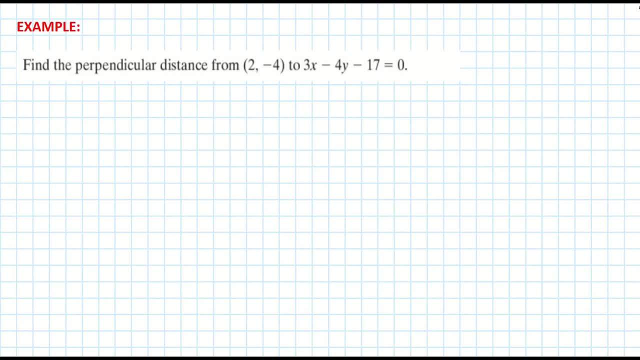 find the perpendicular distance from the point 2 minus 4 to the line 3x minus 4y minus 17 equals 0. So perpendicular distance draws my attention. so to page 19 in your log tables, And we take down our formula. Like every exam question we're doing, we must write down our formula first of all. 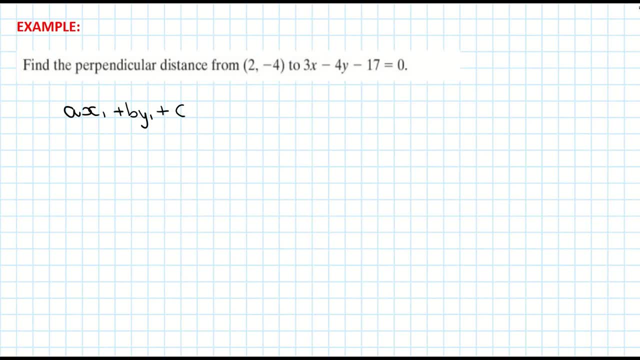 So our formula is ax1 plus by1 plus c, all over the square root of a squared plus b squared On the top of my fraction. I put these into the modulus brackets because that means my answer must be positive. So next thing I would do is I would put my answer into the modulus brackets. 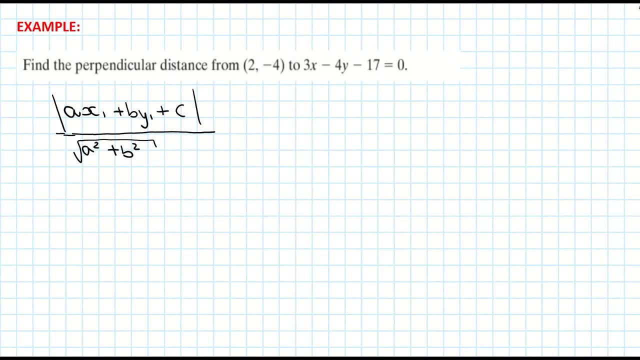 So what I'm going to do is write down the values of my a, b and c before I sub them into my equation. So my a is the number in front of the x, which is 3.. My b is the number in front of the y, which is: 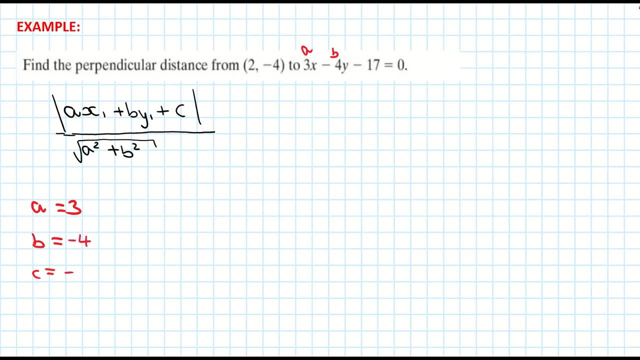 minus 4.. And my c is the constant on its own, which is minus 17.. My x1 and my y1 are my coordinates, So x1, y1.. So now I'm going to fill in my formula. So best thing to do here is to use 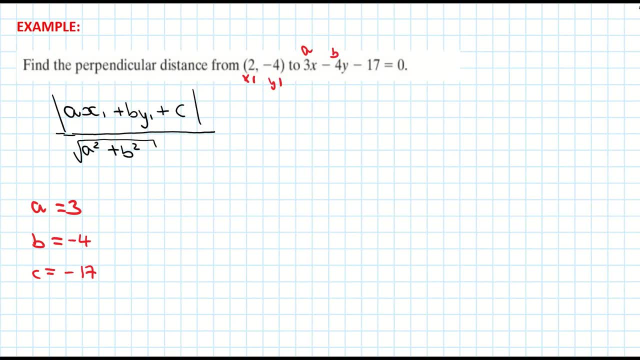 a bracket. So when I'm subbing in my a, just make sure that the 3 is going within a bracket. So it's going to be 3 within a bracket times my x1, which is 2.. The formula then has a plus b, which 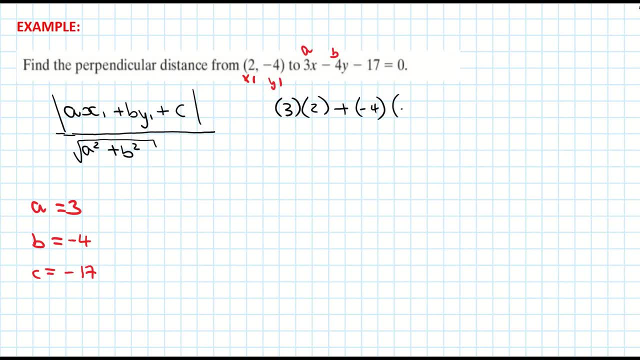 is giving me minus 4 times my y1, which is minus 4 as well, Plus my c, which is plus my constant, which is minus 17.. That's the value of my c. Put in your modulus brackets, and that's all over the square. 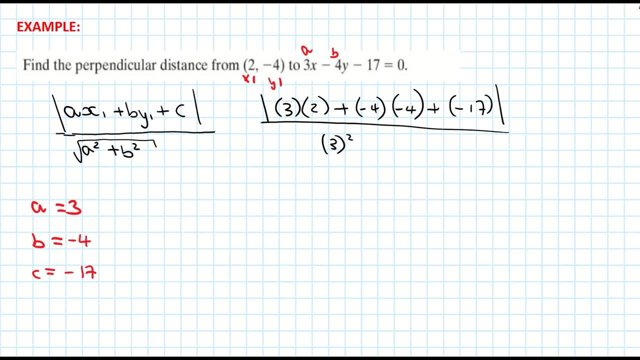 root of a squared which is 3.. So that's the value of my c, Put in your modulus brackets and that's all over the square root of a squared which is 3.. It subway and it tablespoons my b, which is minus 4, plus my b, which is minus four, to be squared. 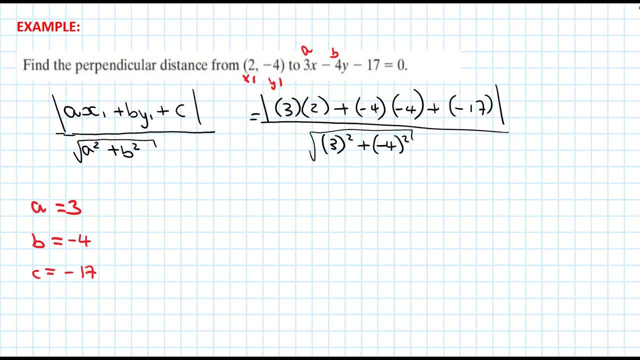 The Understood Lyric, That is the perpendicular distance formula filled in. Let's evaluate it. 3 by 2 is 6 minus 4 by minus 4 is positive 16.. And then plus minus 17 is negative 17 all over. the square root of 3 squared is 3 by 3 is 9.. 4 squared, which is negative, 4 by negative 4. 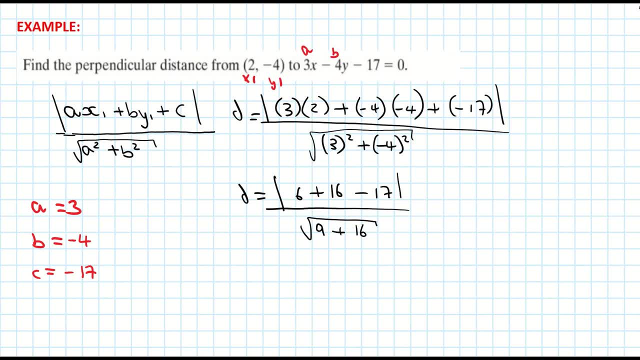 which is positive 16.. Just arrive at the area of y squared from the square, So remind yourself particularly of the Hin hoch. This will get you as much better. will it just be careful, if you're using a Casio calculator there, that that goes into? 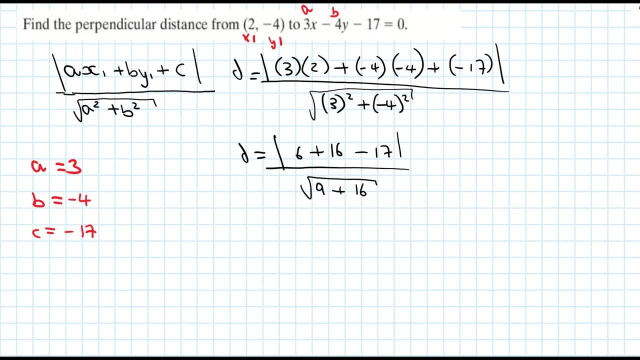 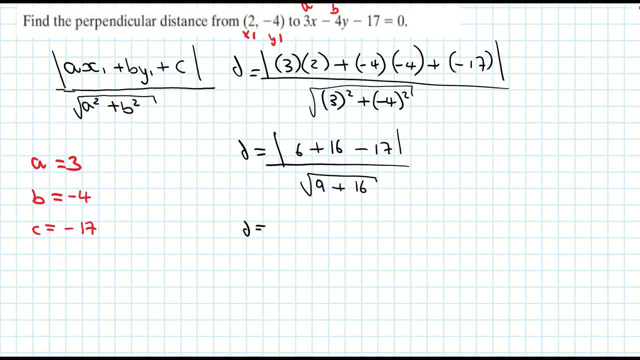 brackets, otherwise your calculator will give you a negative, which we don't want. adding the top line, we get distance is equal to 6 plus 16 is 22. take away 17 is distance of 5 over the square root of 25. so D is equal to 5 over square root of.